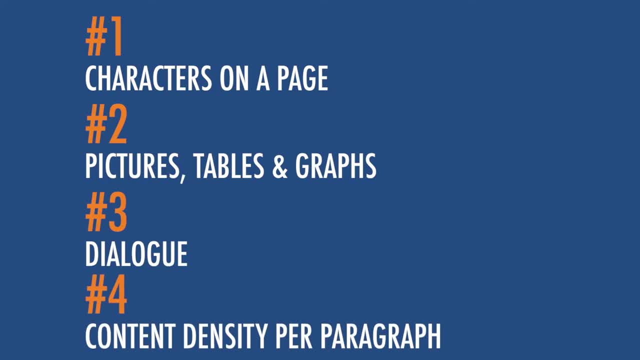 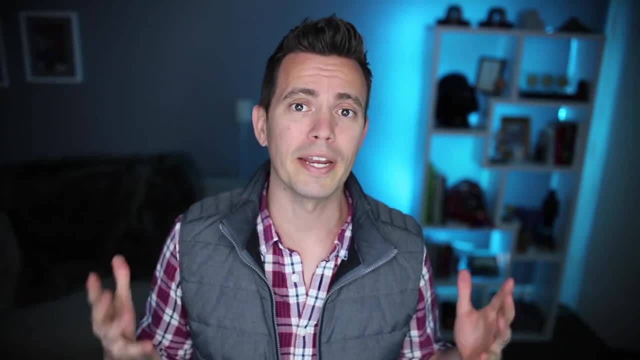 of different paragraphs for it, or if you write in a type of genre that has very thick content, density per paragraphs, like legal books and things like that. So exactly how can one answer this question? Well, we found a way at Kindlepreneur. But before we do that, if you like videos like 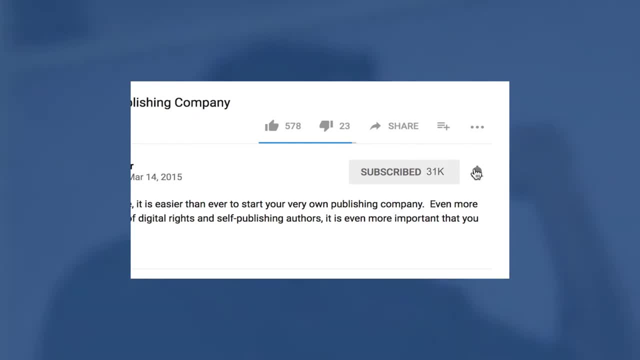 this and would like to learn more about book marketing. please subscribe to our channel And, if you like book marketing, go ahead and hit the subscribe button as well as the little bell icon, so as to get a notification when my next video comes out. And with that let's begin. 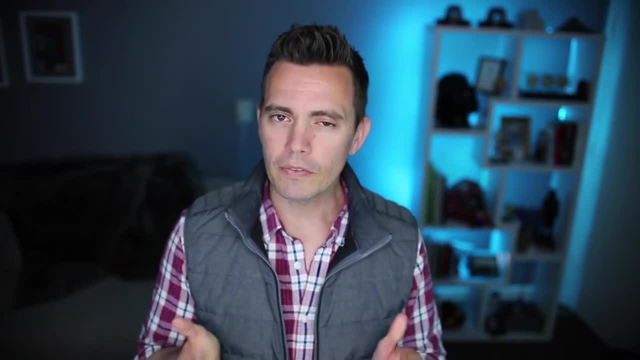 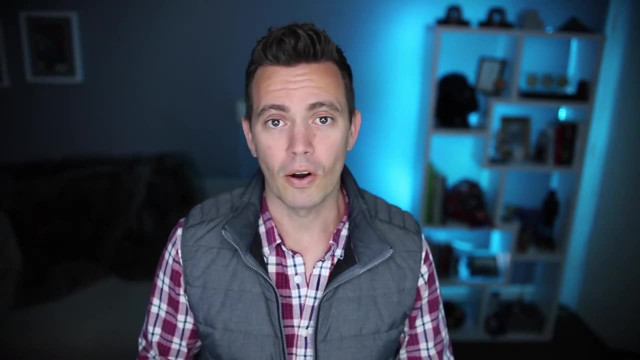 Okay. so, since there are so many different factors that affect this and everybody's looking for kind of a rule of thumb to use in order to, shall we say, figure out what their book may equate to, we surveyed our email list at Kindlepreneur and thank you to all the people that filled in. We had 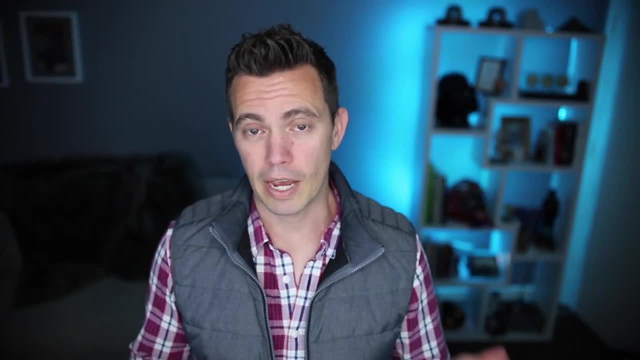 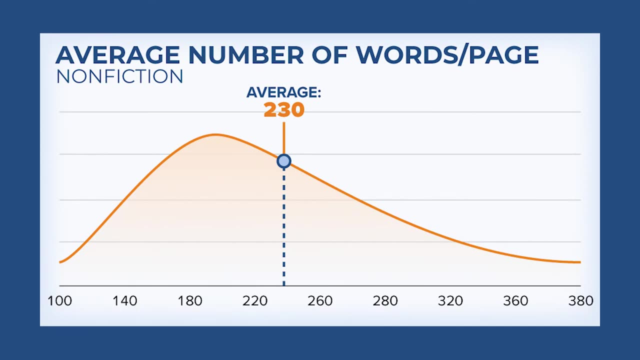 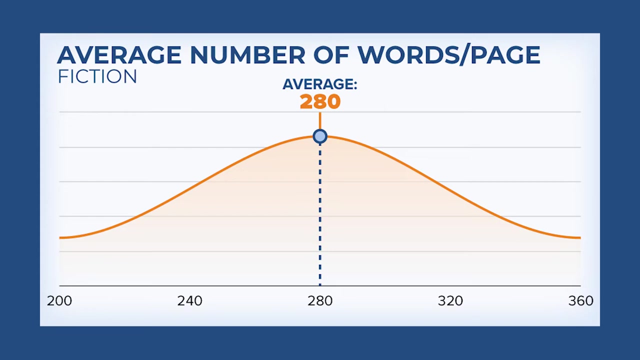 over 1,800 responses. Using the information that we got from that survey, we broke it down into two graphs. The first is fiction and the second one is nonfiction. Taking the average of the information we got from fiction, we saw that you can expect about 280 words per page on Amazon Kindle With nonfiction. 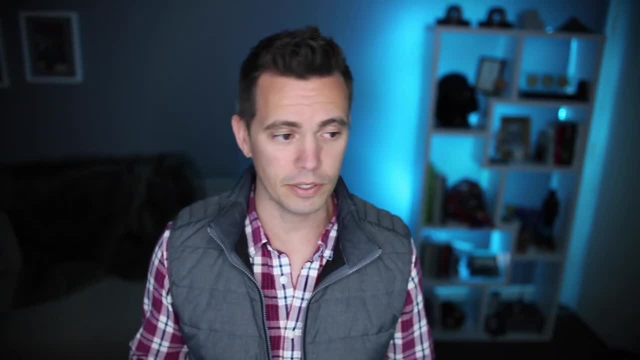 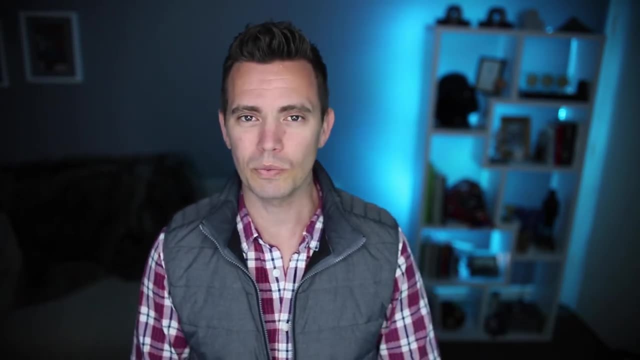 it's 230 words on average. Now again, as you can see from these graphs, it can vary greatly depending on just your writing style and all the other things we talked about, But you can use these numbers as a really good rule of thumb in trying to guess at how many pages Amazon will choose for. 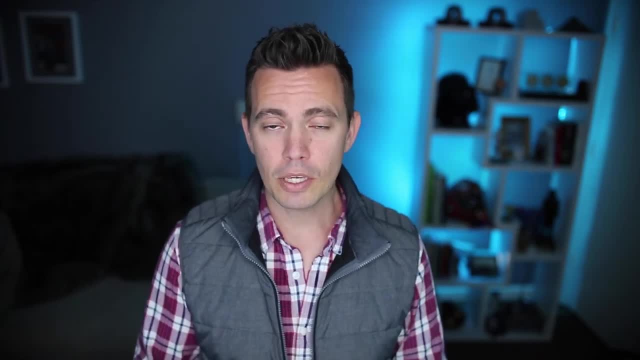 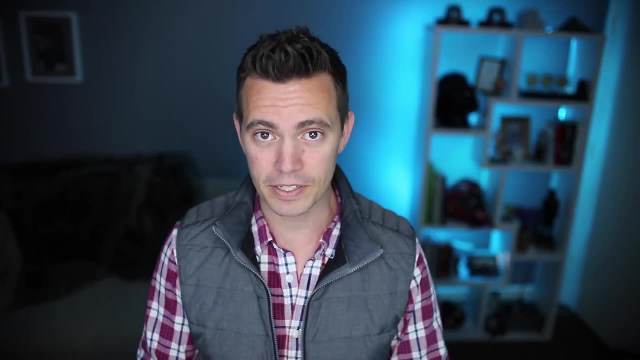 your Kindle book Now. an important note to make, though, is that the moment that you upload a physical book, Amazon will usually take the physical book number of pages and use that for both the physical and your ebook. However, if they don't and you 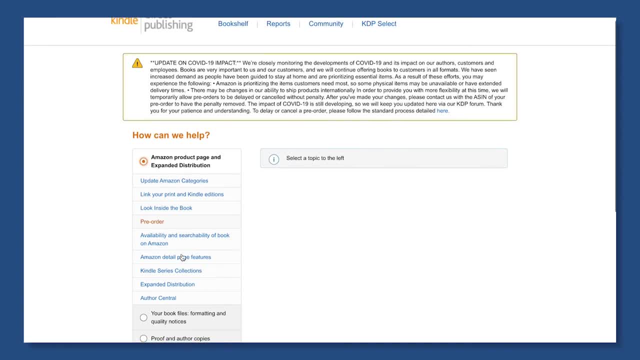 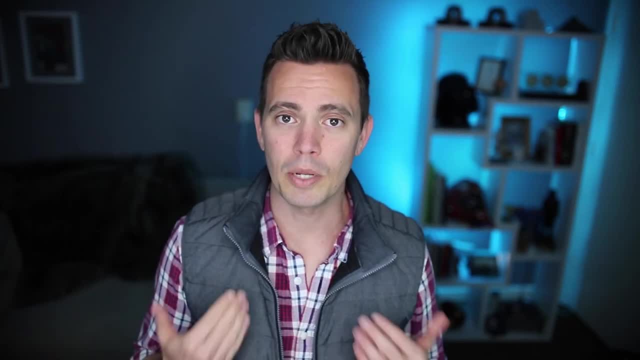 want it to reflect your physical book, make sure to contact support. They'll change that up. lickety split for you. Okay, guys, there you have it. Using this rule of thumb, you can now guess at how many words per page your book could be taken with Amazon. So, whether it's fiction or nonfiction, And with that we'll see you in the next video. 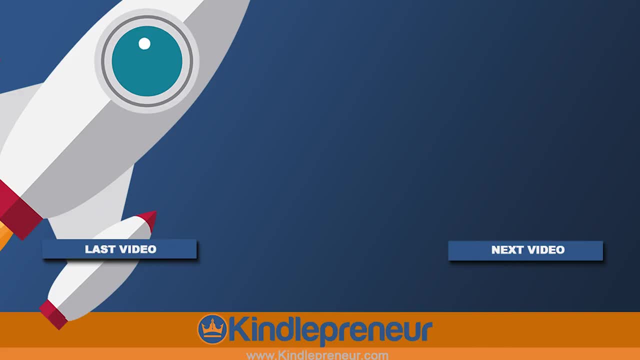 With that, I'm Dave Chesson of Kindlepreneur signing off Cheers.